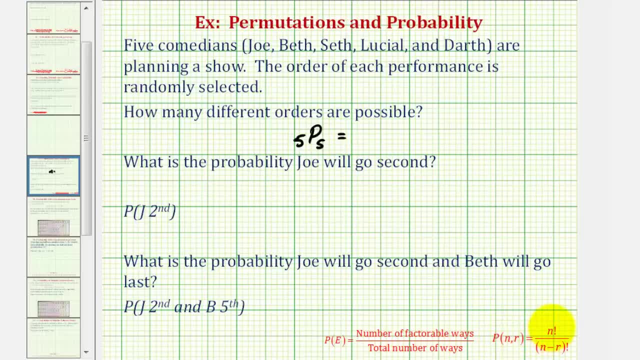 Either way, n permute r is five permute five r is equal to n factorial divided by n minus r factorial. So in this case we would have five factorial divided by five minus five factorial, zero factorial. Well, zero factorial is equal to one. 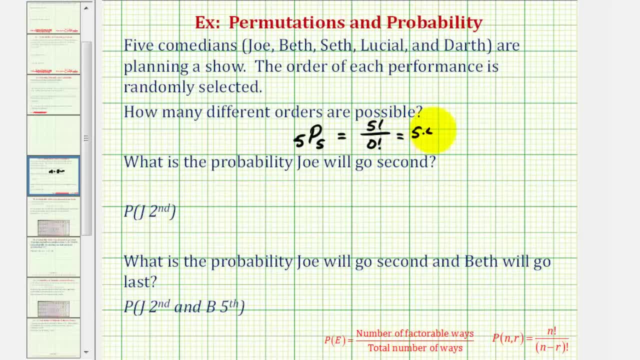 So this is just equal to five factorial, or five times four times three times two times one, which is equal to 120.. So there are 120 different orders possible. Let's also take a look at this using the counting principle. For the counting principle, we view this as a series of events where 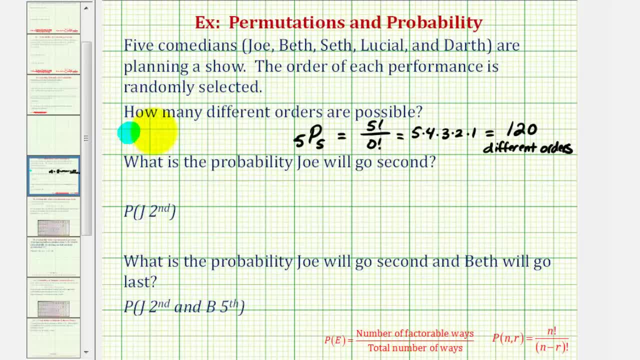 since there are five people being ordered, there would be five series of events will determine the product of the number of ways each event can occur. So, for example, anybody can be first or any of the five comedians. So there are five ways we can select the first position. 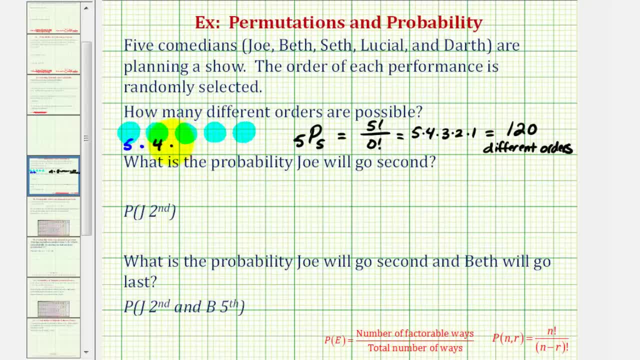 There are four ways to select the second position. There are three ways to select the third position. There are only two comedians left, so there are two ways to select the fourth position and one way to select the last position. Notice how this product would be five factorial, giving us the same result. 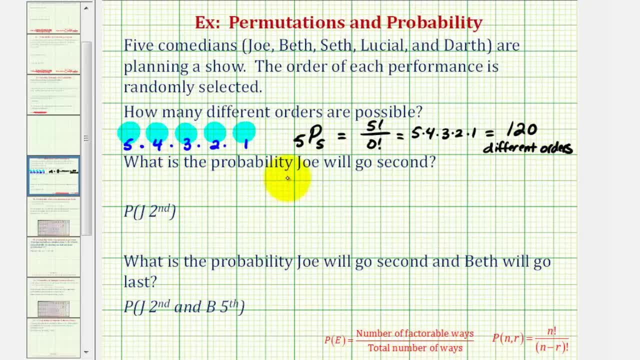 And now for the second question. we want to know what is the probability. Joe will go second. Again, we can use a permutation, or we can also use the counting principle. But either way to find the probability, we want to find the number of favorable ways this can occur. 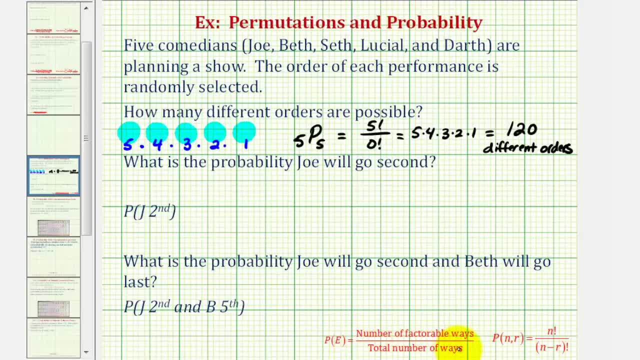 and divide by the total number of ways we can order the comedians. So if there are five positions to fill and we want Joe to be, second notice- there are only four positions to be filled and therefore the favorable number of ways this can occur would be: 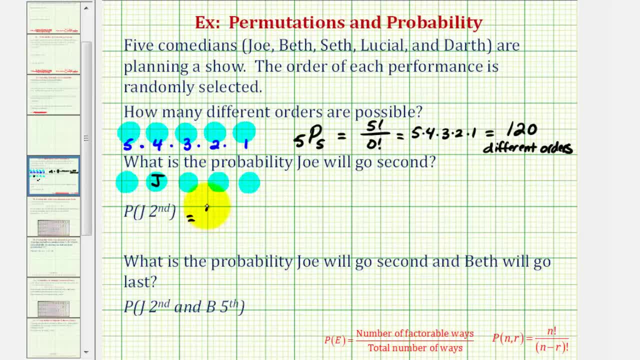 by permuting the four remaining comedians. So four permute four would be the favorable number of ways that Joe would be second divided by the total number of ways that we can order the five comedians, which we already know is one hundred twenty. 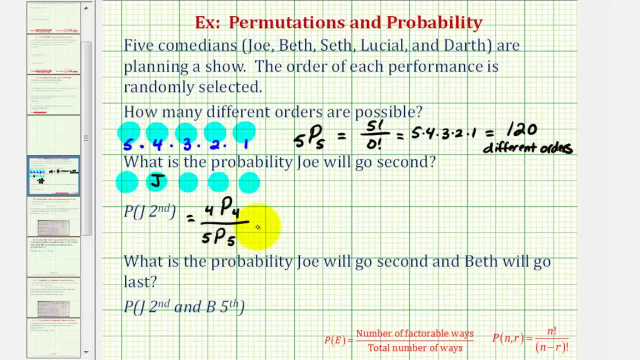 which would be five permute five, which we already know is one hundred twenty For four permute four. by definition, that would be four factorial divided by zero factorial, or just four factorial four times three times two times one, which is equal to twenty-four. 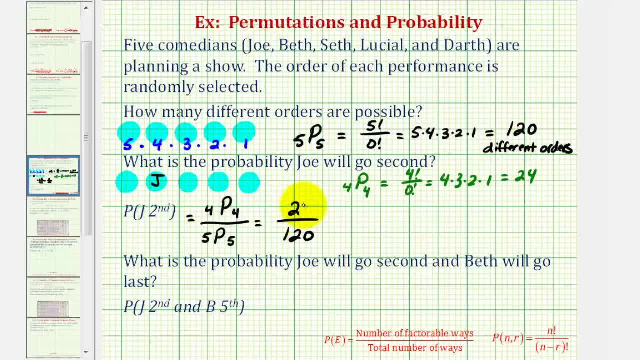 So the probability of Joe being second would be twenty-four over one hundred twenty. But this does simplify. This is both divisible by twenty-four, So this simplifies to one-fifth. Probability can be expressed as a decimal and a percentage as well. 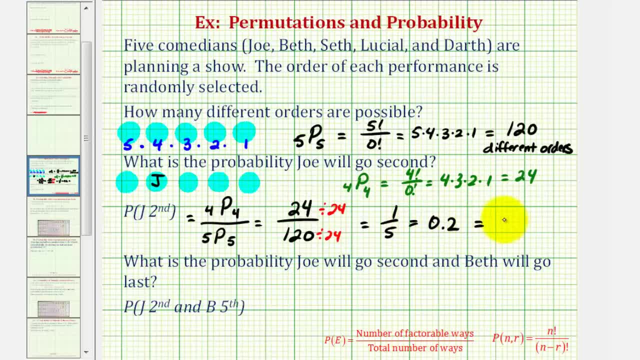 This is also equal to zero point two or twenty percent. But I do want to go back to the counting principle just for a moment. If we know Joe is second- and there's only one way that can occur again if he is second- 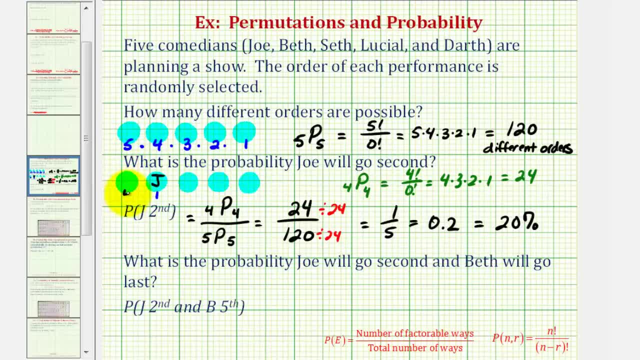 leaving us with four options for the first position, three options for the third position, two options for the fourth position and one option for the fifth position. notice how this would be four factorial or twenty-four, the same as four permute four. 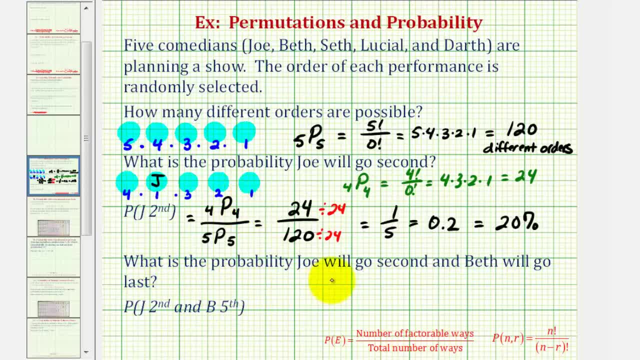 Finally, for our last example, we want to know what is the probability. Joe will go second and Beth will go last. So again, we have five positions. We want to know the number of ways that Joe can be second and Beth can be last or fifth. 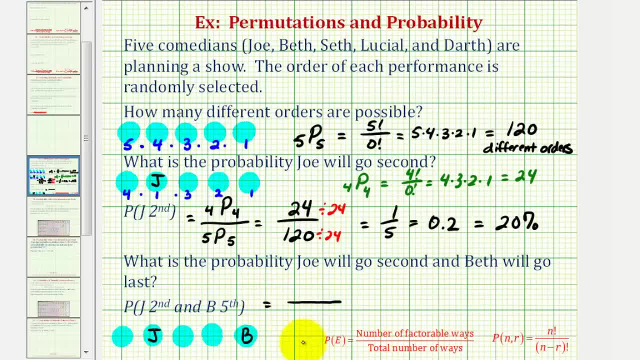 So first, using permutations, the favorable number of ways would be the number of ways we can fill in for the remaining positions. There are three comedians and we want to order all three of them, So that would be three permute three. The total number of ways is still. 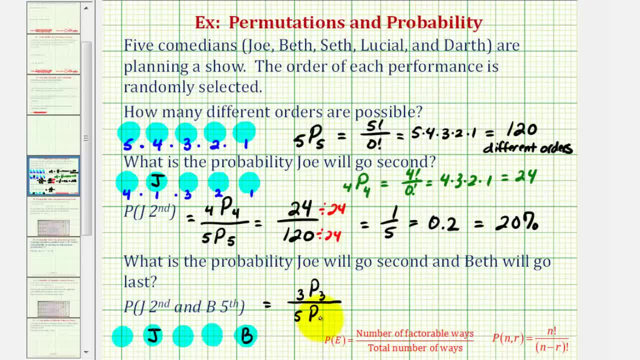 one hundred twenty or five permute five, So our denominator is one hundred twenty. And again, three permute three is equal to three factorial divided by zero factorial, or three times two times one, which is equal to six, And this fraction simplifies as well.